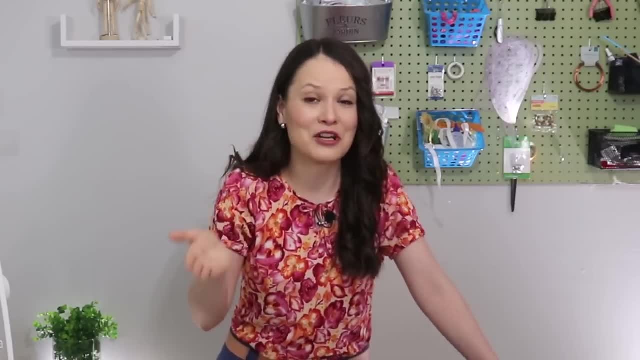 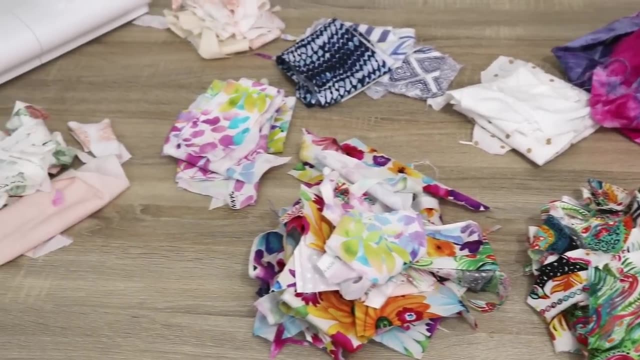 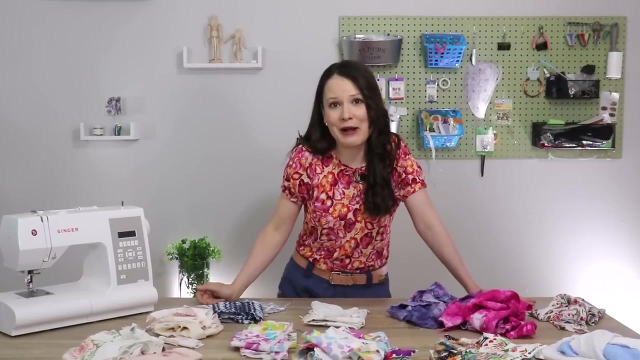 with all of this. But today we're going to turn that frustration into creativity and I have prepared for us six really fun and useful- as you know, that's pretty important to me- projects that we can make for ourselves, maybe as gifts, even to sew and sell, if that's something that you're into. 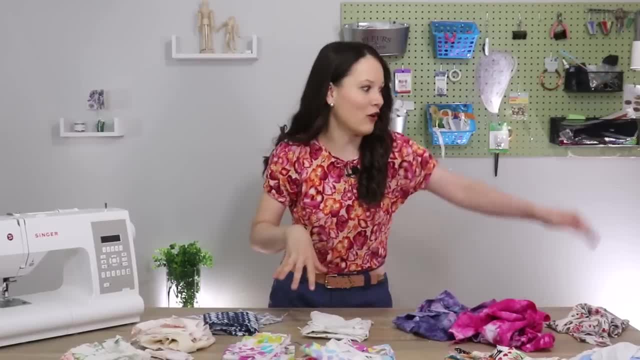 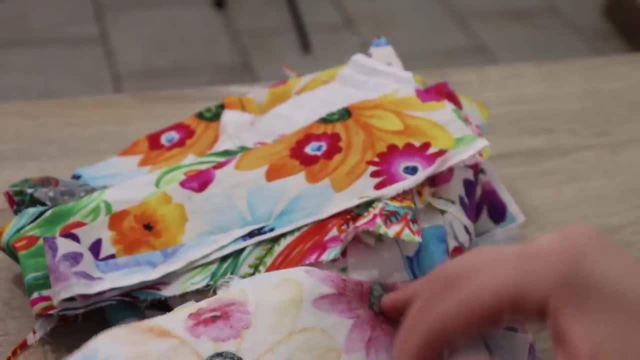 And here I have all sorts of different fabric scraps, and that's not even all. I have some extra, As I said, they do appear out of nowhere, and here you can see all sorts of different colors, all sorts of different prints and different sizes, from like really tiny ones to a little. 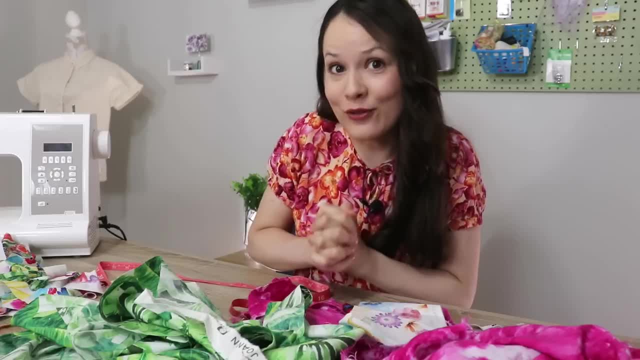 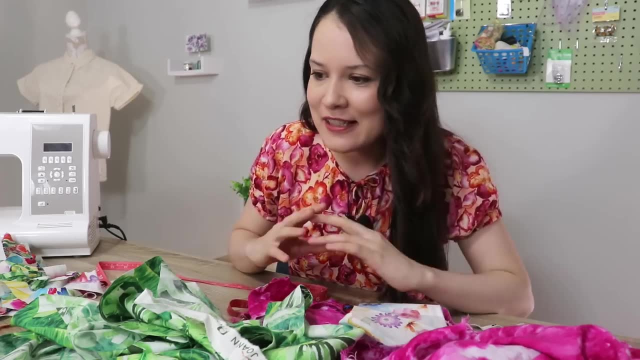 bit bigger. So I think we're going to have a lot of fun today, All right, so first things first, let's talk about fabric. And for me, and possibly for you as well, when I'm working on smaller fabric projects, it's kind of a no-brainer, you just you know. 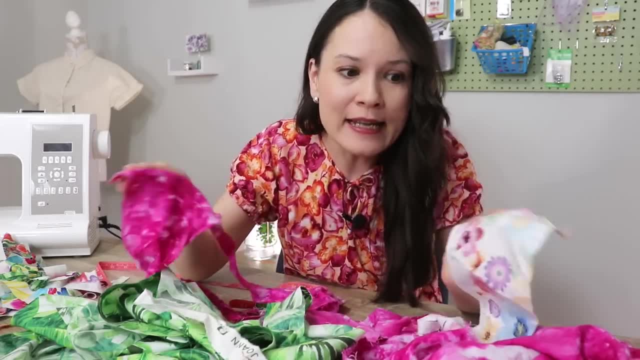 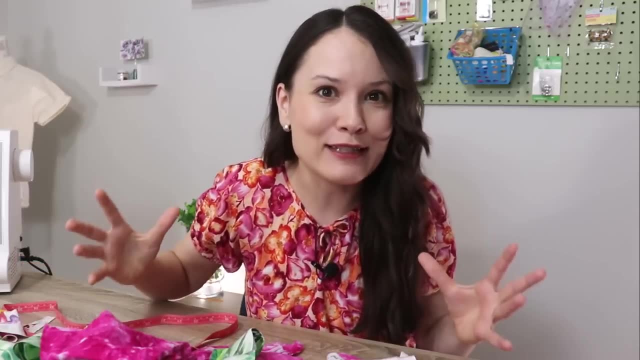 you pick a piece that is big enough for what you need and you get going right Now when I need a larger piece and I don't have it, but I want to use my fabric scraps for it. I feel that that's where things start to hit the wall, because it can be sometimes a little. 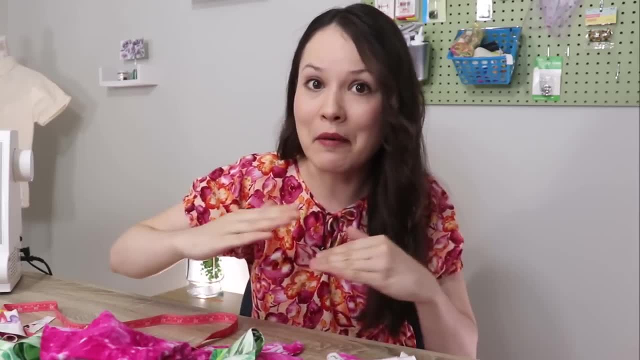 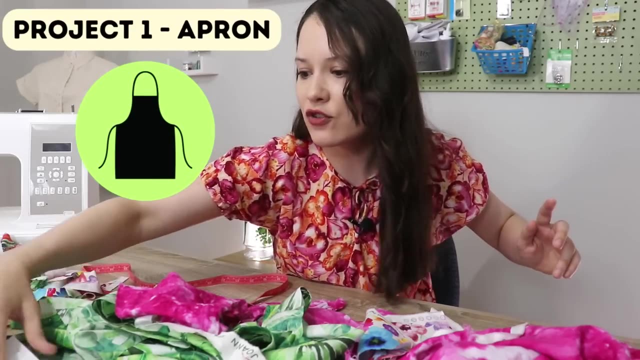 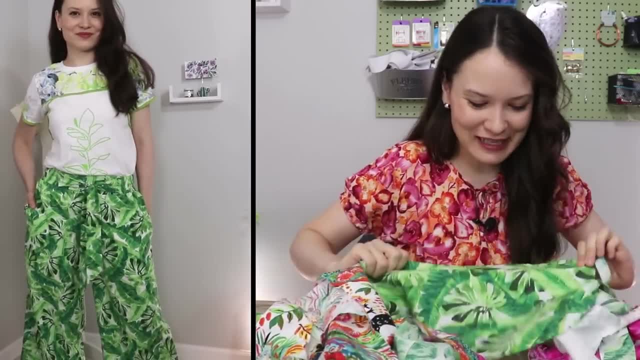 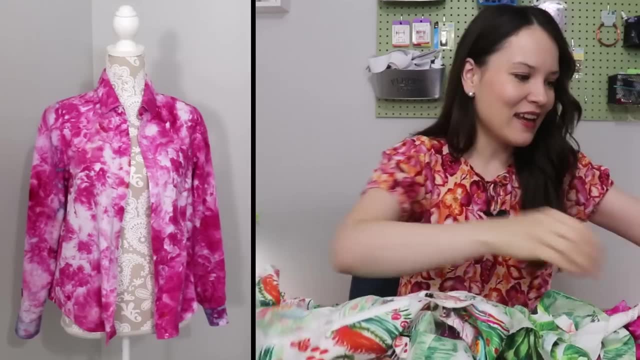 And here I have some beautiful fabrics from all of the past projects that you've seen. You remember the pants that I made from this cotton. You remember the blouse that I made from this cotton. I also made a button-up shirt from this juicy, bright pink. Of course, I made a 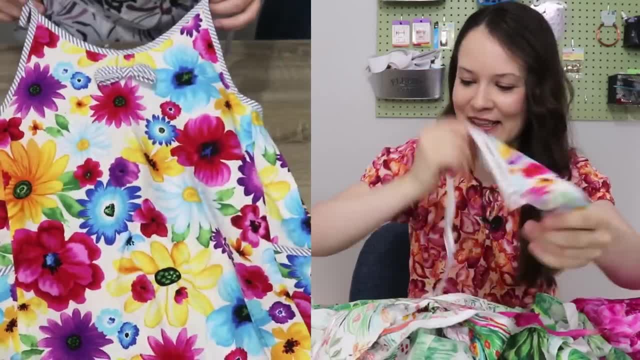 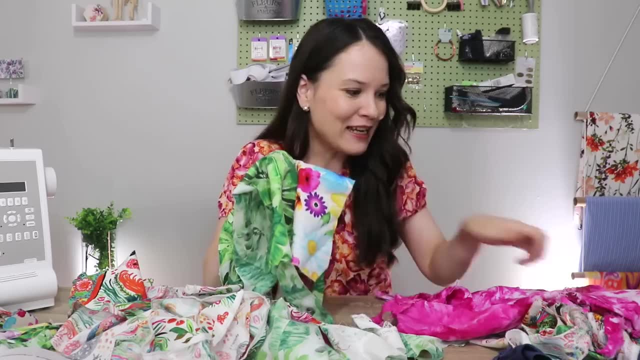 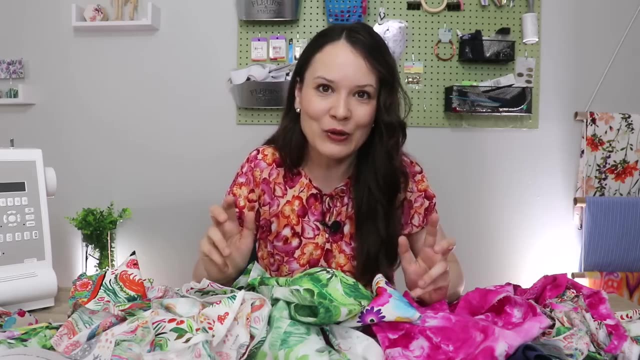 lot of dresses for dress a girl around the world from this cotton and it might seem like all of these really don't go together, but I think if we combine them strategically it could actually look really well. I think the key, at least for me, is not to be afraid of all those juicy colors. 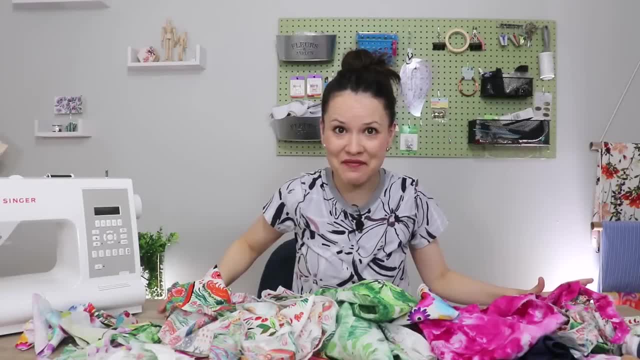 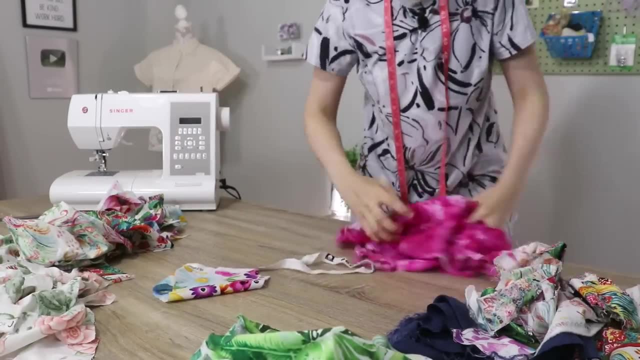 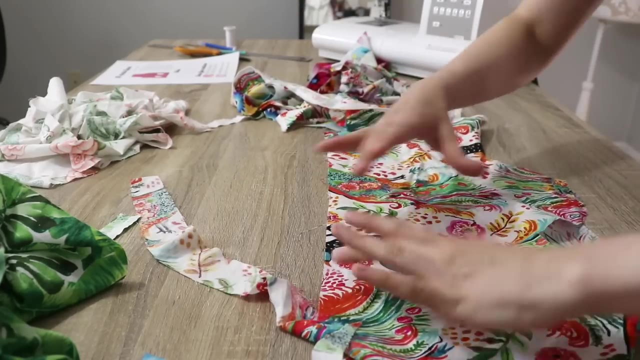 and just sort of embrace them. Okay, I'm ready Now. first I'm going to take a look at what fabric scraps I have and which ones are going to be the best for this job, And I want to stick to natural content of sturdy fabrics like cotton and linen. From looking at what I have here and the shape of 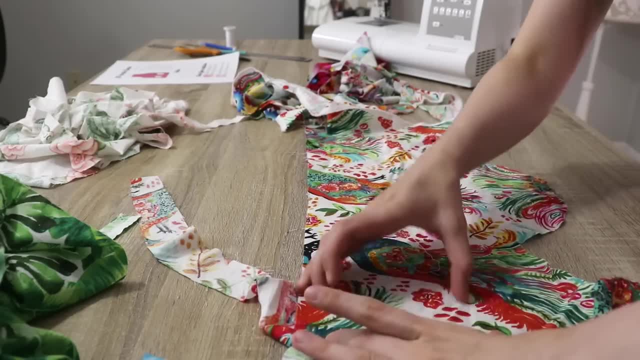 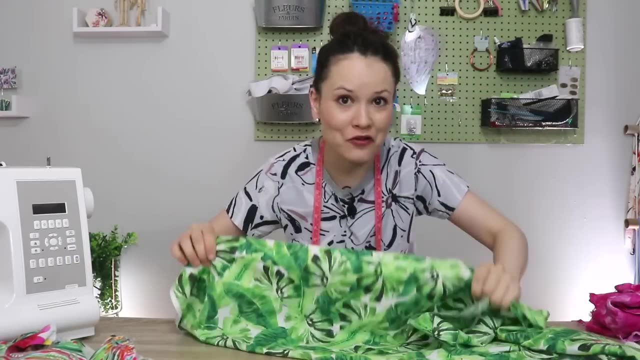 the fabric scraps. I think the best case scenario for me would be to go horizontally, so to make my yardage from strips of fabric. And looking at this tropical cotton now, I actually want to stretch it for two projects, but since I have a bit more of it than any other fabric scraps, I think this is 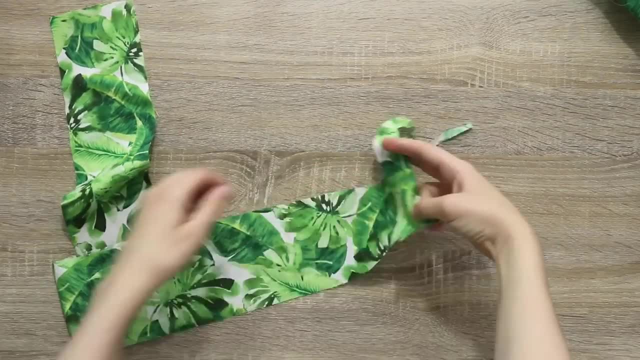 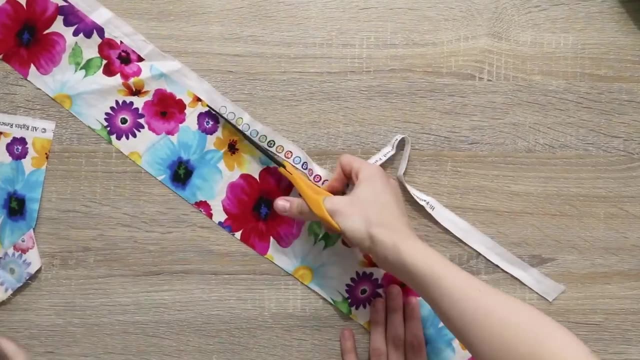 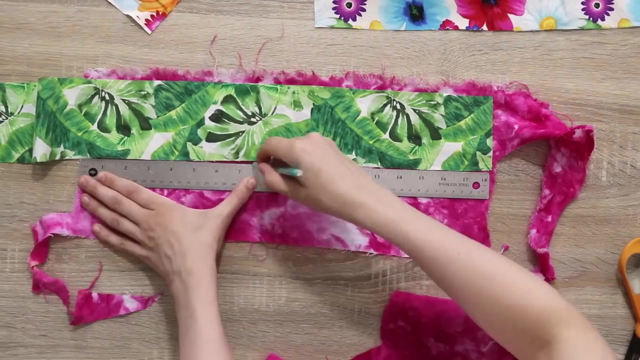 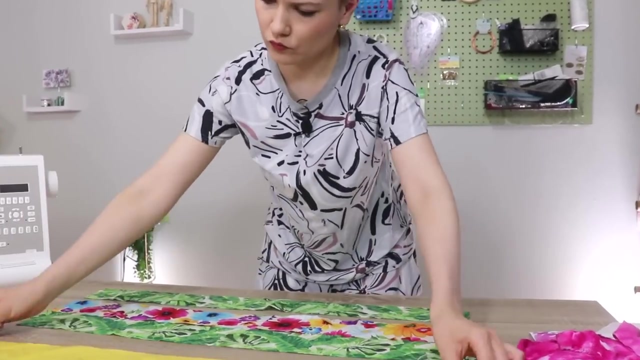 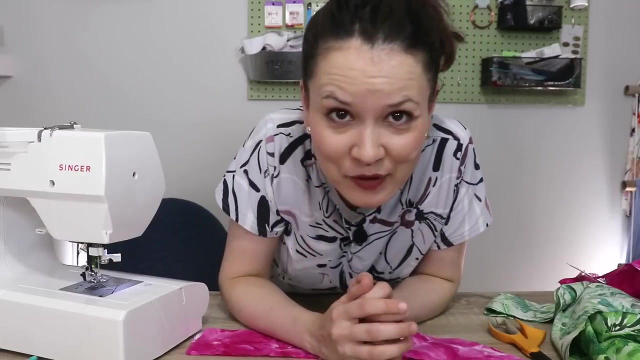 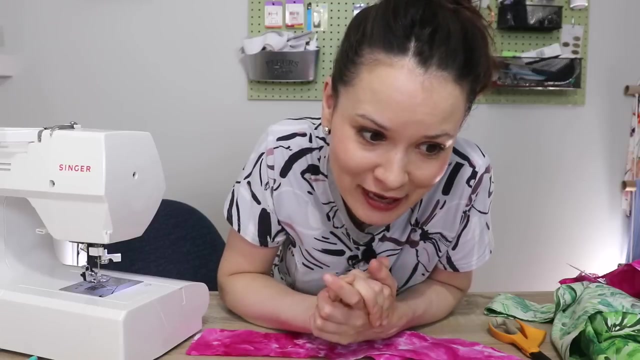 going to be the lead in my composition. So sometimes, with the projects like this, I feel that the best thing to do is not to overthink. So I'm just going to start at somewhere where I have enough fabric for the entire project. So we're just going to see. 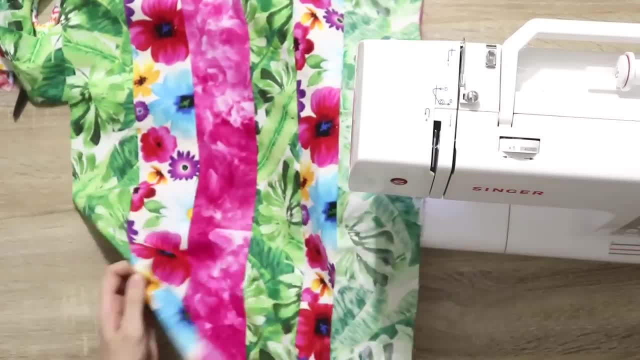 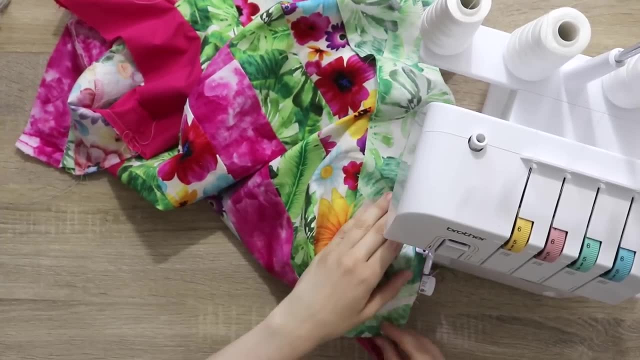 The method of construction here is really simple and straightforward. I'm using just 3 eighths of an inch seam allowance, or about one centimeter, and doing a straight stitch first, which I then finish with a serger. Okay, so it's coming together. I'm going to start with the bottom of the bag, So I'm 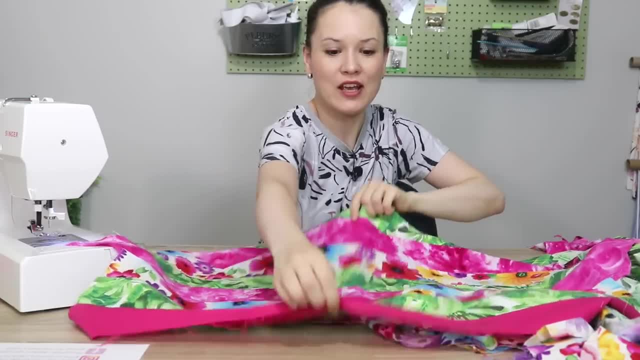 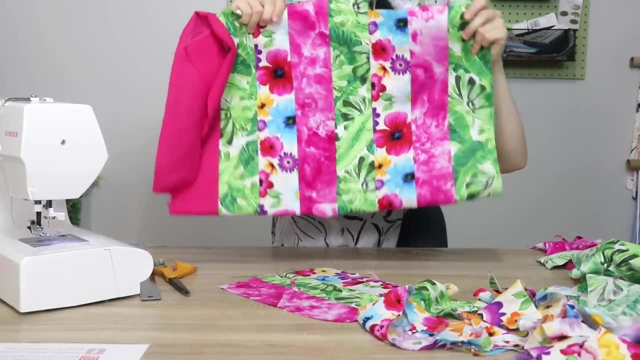 actually really liking the results. So at this point you could turn it into like a throw pillow. You can also turn it into a tote bag or beach bag. You can turn it into so many different things, but, as you have gathered, I'm working on an apron. 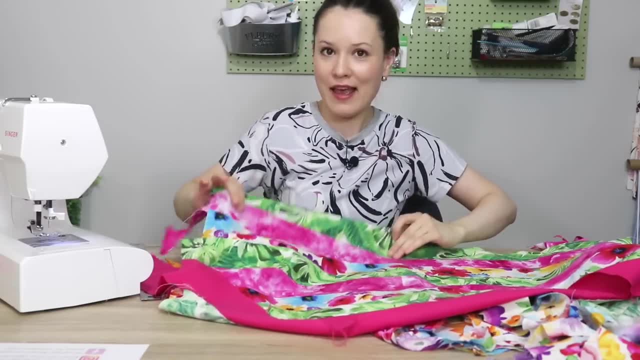 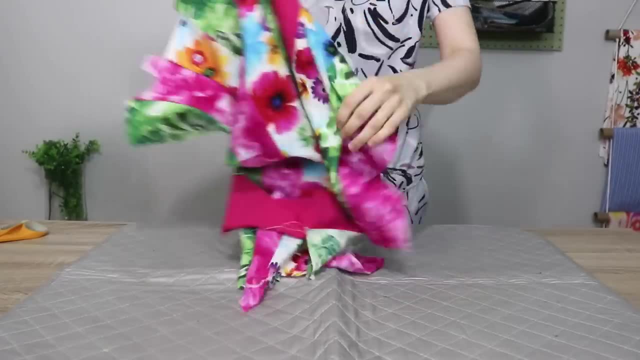 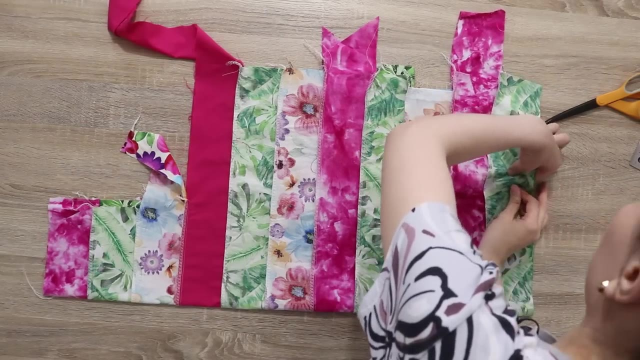 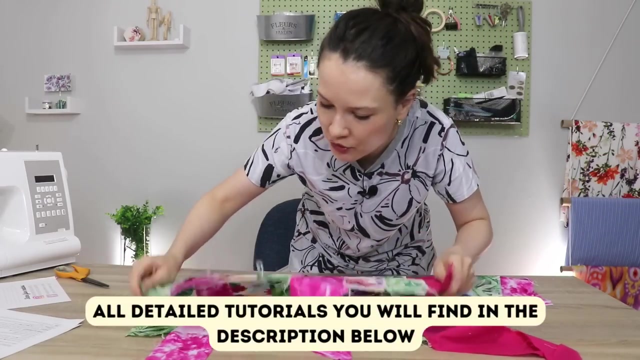 So I also have to figure out the top part of the apron and then assemble everything else. Now I'm just going to fold it right sides together and I will cut my apron shape out of it. I'm just going to do it right on fabric, referencing the measurements that I have. 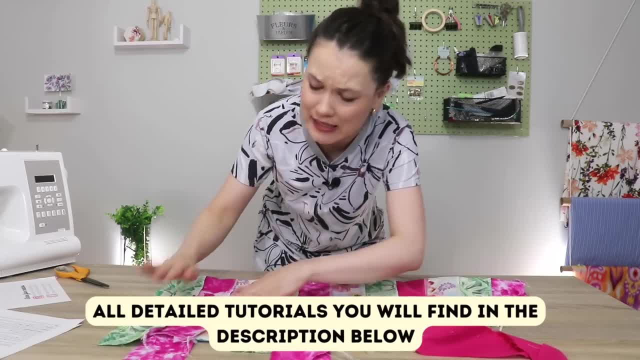 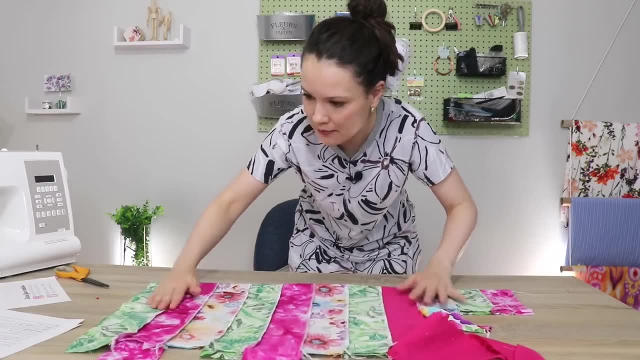 Of course, if you're not sure, then definitely make a pattern first. It's really easy, really straightforward: All measurements you already have. All you got to do is just make an actual pattern- But I'm going to do it right away- and then a few final steps and we'll be ready. 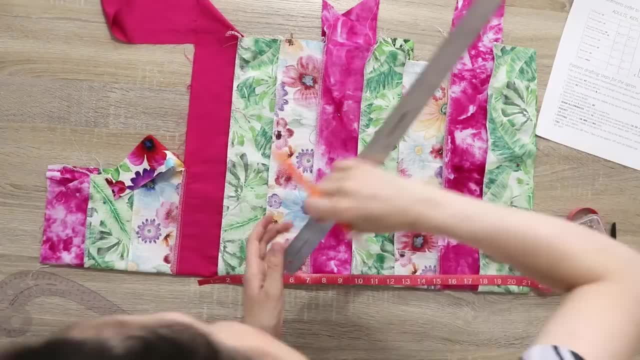 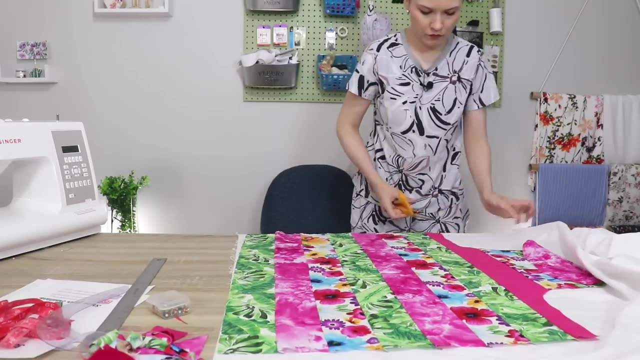 Now, in the original sewing and drafting video for an apron that I have on my channel, the final steps are as easy as hem the apron and add the straps. But since I'm working with fabric scraps here, I decided to take a different route. 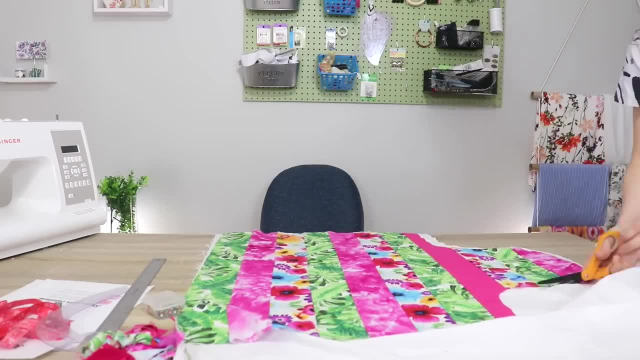 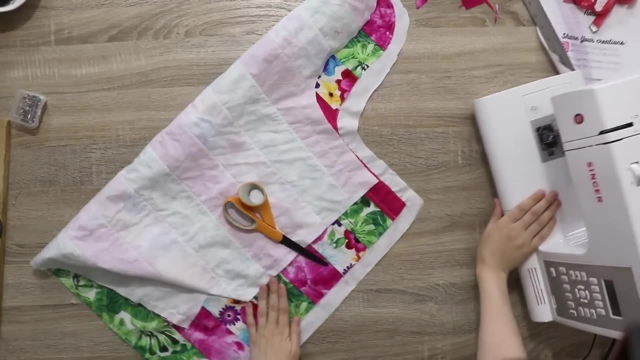 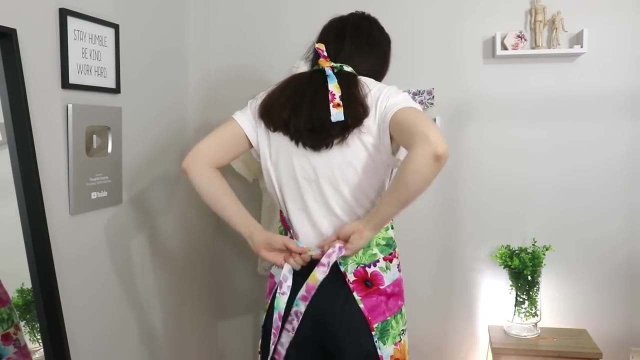 So first I added a light cotton backing to this apron. It's just a piece of cotton that I decided to top stitch to create this fabric sandwich. Then I actually went ahead and rounded all of the corners of my apron and finished the raw edges with a bias tape. 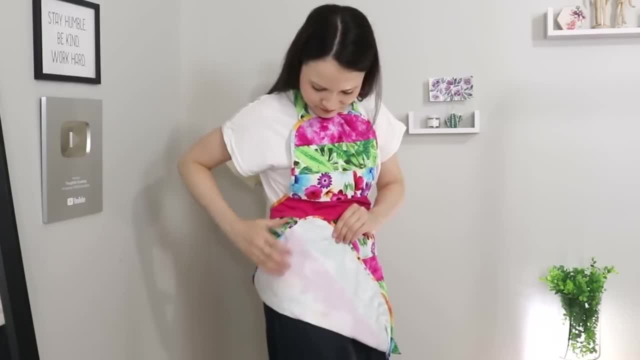 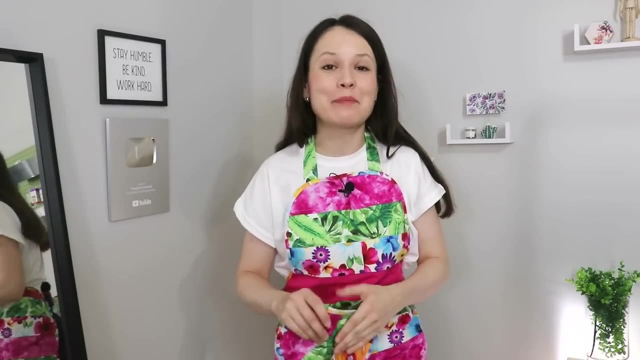 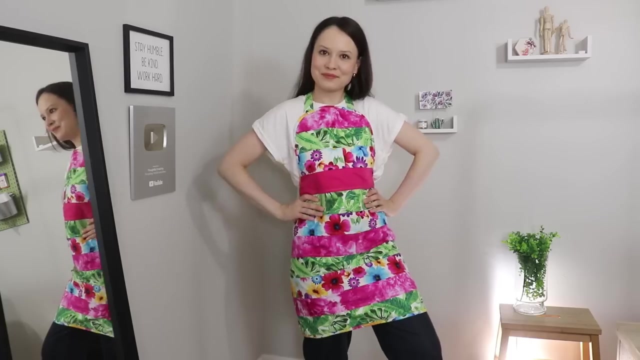 Now, as always, you don't have to like what I created, but I truly hope that this experiment inspired you to use up your fabric scraps and to create that yardage for bigger projects that you have in mind, And perhaps you're going to go for something more monochromatic. 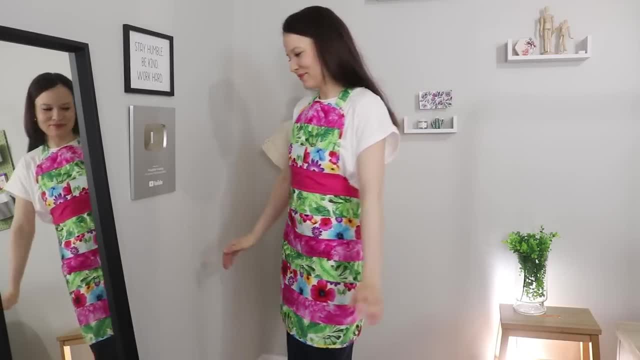 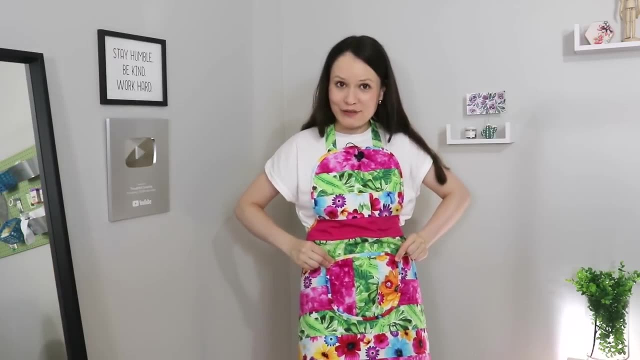 maybe tone on tone, Maybe you will use solids and patterns of the same color combinations. Just do what's right for you. I also made a little pocket that's going to go right over here. I'm going to make a little pocket that's going to go right over here. I'm going to make a. 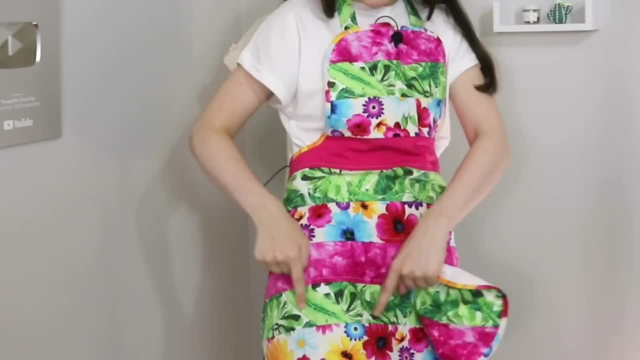 little pocket that's going to go right over here. I'm going to make a little pocket that's going to go right over here And, as I mentioned, I was planning to squeeze out one more project out of this green fabric and that is going to be great for all those tiny little fabric scraps. 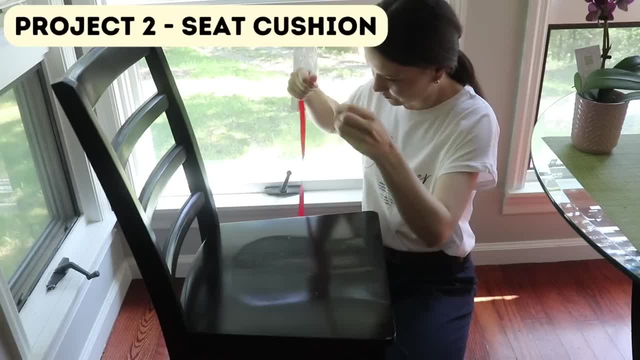 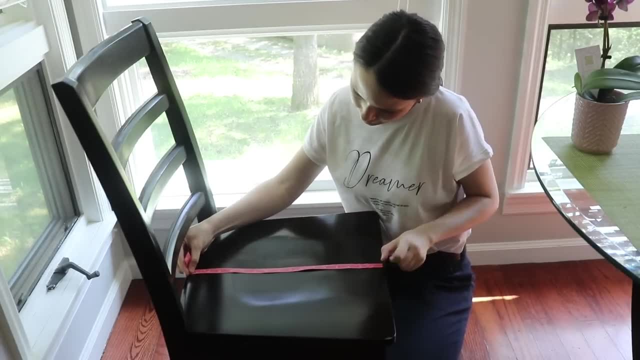 that you have, and also for those decent fabric scraps as well. But first I got to take the measurements. Here I'm going to be creating a seat cushion for a chair for my little one, so that way she can sit in the big girl chair and actually reach the table as well. 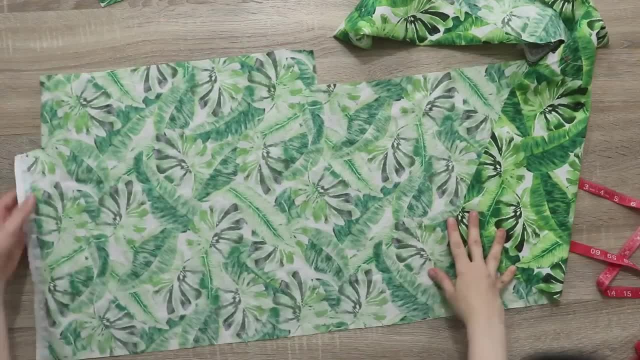 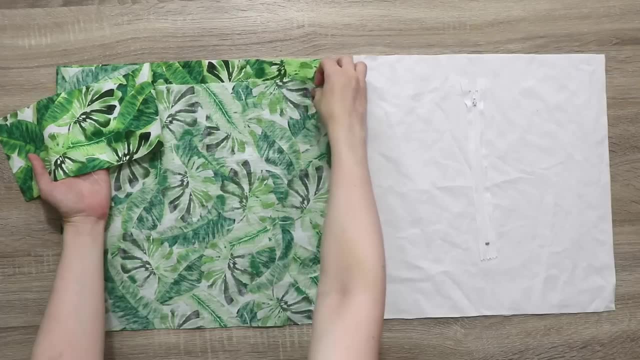 The measurements that I got was 16 by 16 inches, so we'll see what we got here. The measurements that I got was 16 by 16 inches, so we'll see what we got here And if we can work around it Now. I managed to cut one solid rectangle from the green fabric, and one that 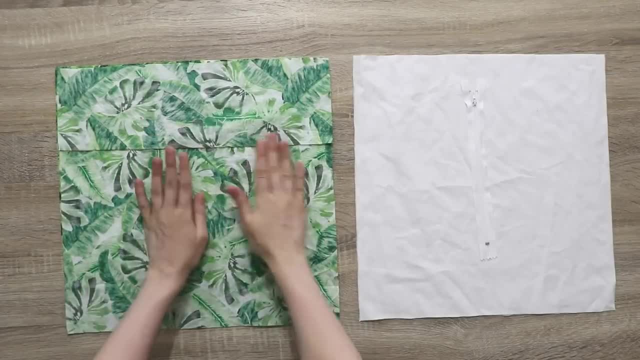 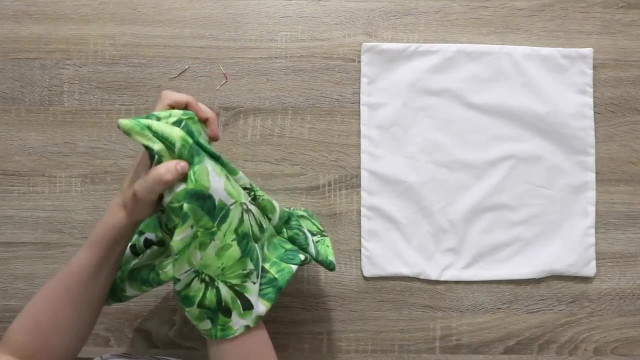 was combined from two pieces overlapping each other, which actually works great, because I'm going to be making an envelope cushion And, by the way, as always, I have all of these detailed tutorials on my channel. so right now we're going to be focusing on the concept itself. 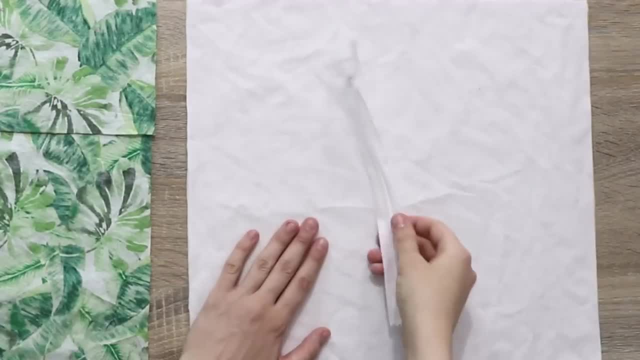 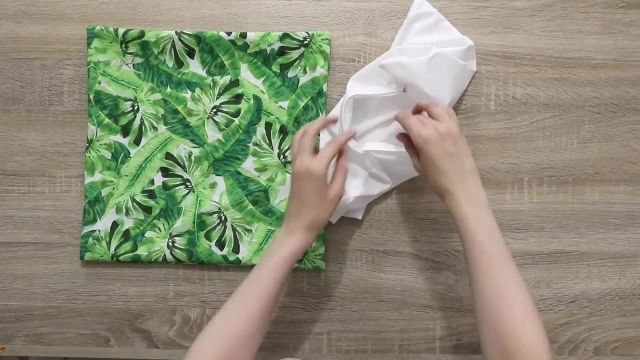 Now the second cushion is going to feature a zipper and is made just from white cotton fabric, the same one that I used for backing the ear. Now the second cushion is going to feature a zipper, the same one that I used for backing the ear, Once the insert for the cushion is ready. 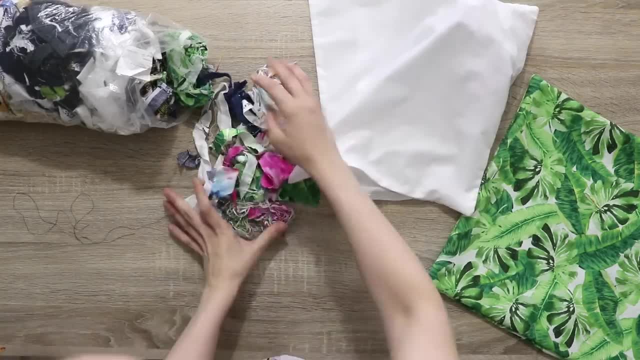 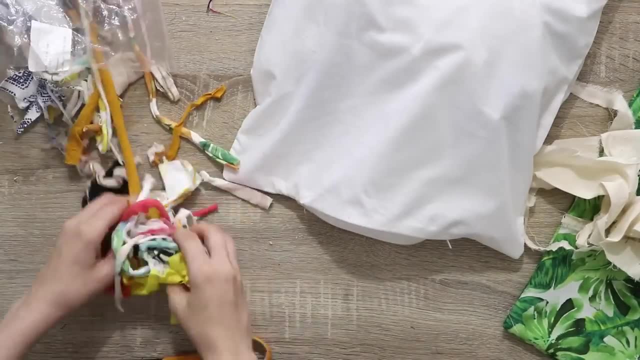 for me. that's the white one with a zipper. I just go ahead and stuff it with all the little fabric scraps that are no longer good for any other project. And yeah, to be honest, because it's going to be a butt cushion, a seat cushion, I don't actually need it to be. 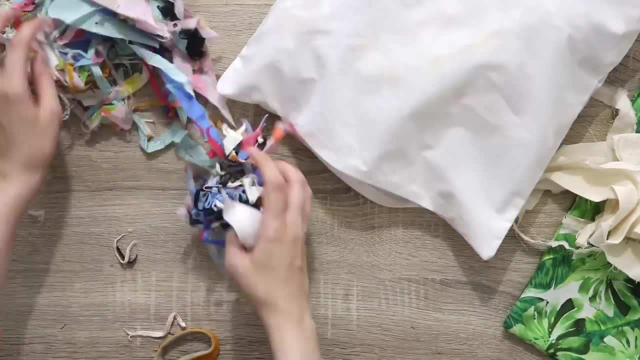 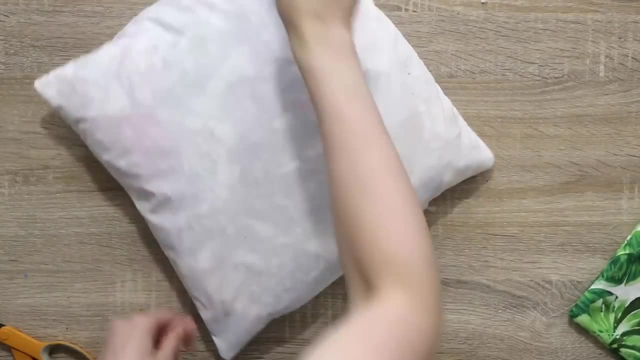 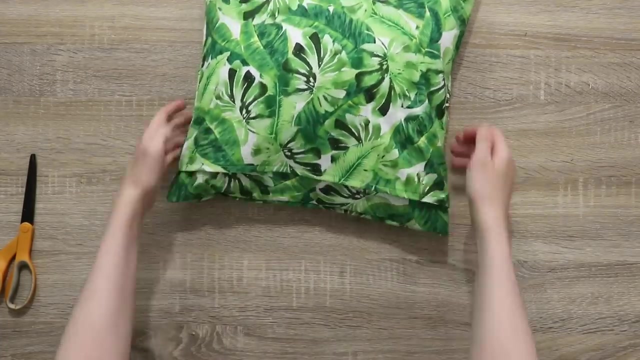 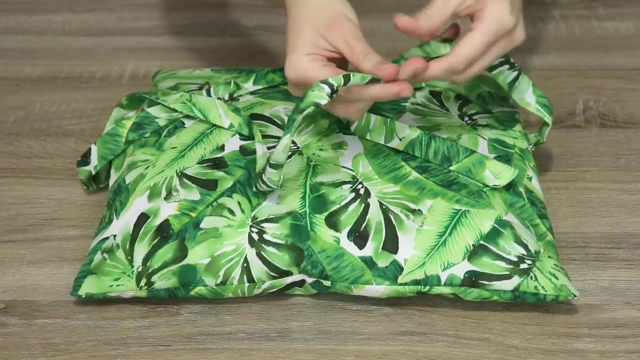 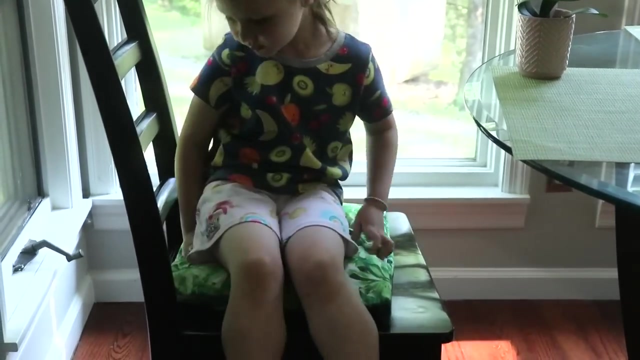 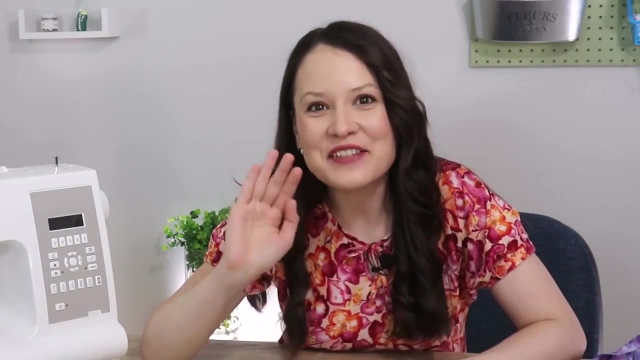 super fluffy and soft. I prefer for it to have a little bit more thickness to it, so that way it actually serves the purpose. And then I added two little ties and the moment of truth. let's test it out. The main point is to have fun. Are you having fun? If you are having fun, 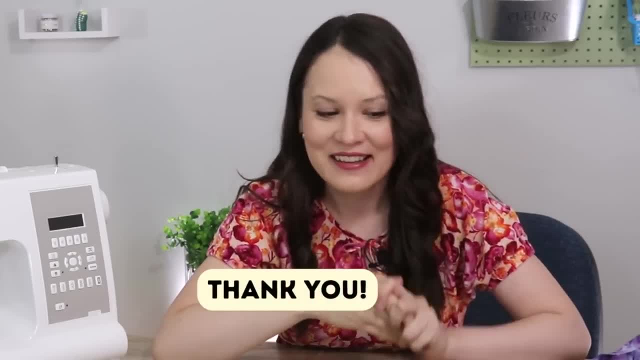 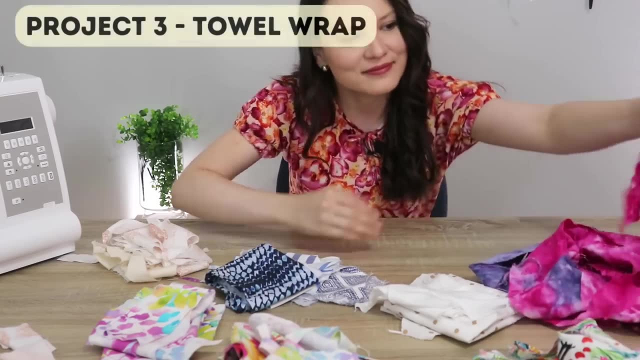 give this video a thumbs up so that way, I know that you're with me, and I truly hope that this video gives you a ton of ideas. This next one will come in handy if perhaps you have some extra towels that you don't use, or if you're like me and you have some towel and fabric scraps. 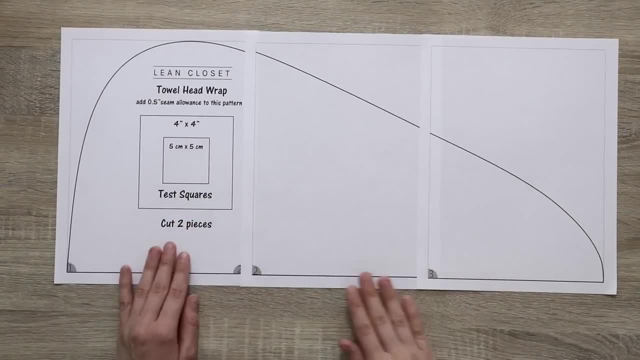 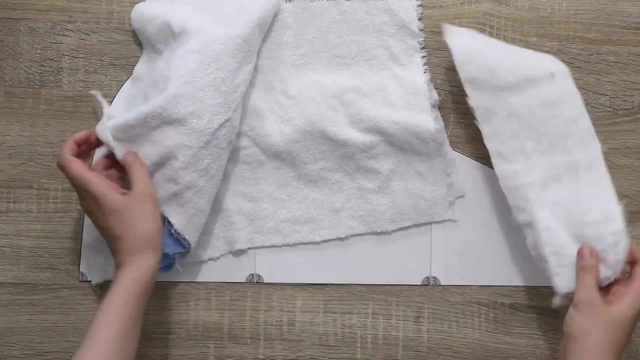 I am starting with assembling my pattern, but of course you can draft your own as well. as you can clearly see the shape of what we're going to be making on your screens. I have just a little bit of this blue and white toweling. 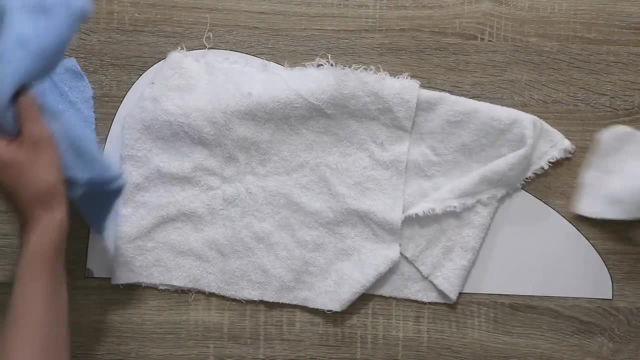 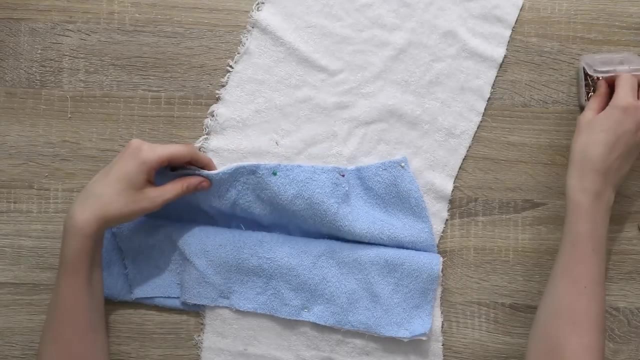 and neither one of them is enough in order to make a full towel head wrap. first I figure out what would be the best way to arrange my fabric scraps, and then I combine them using the same method as I did in the first apron project. 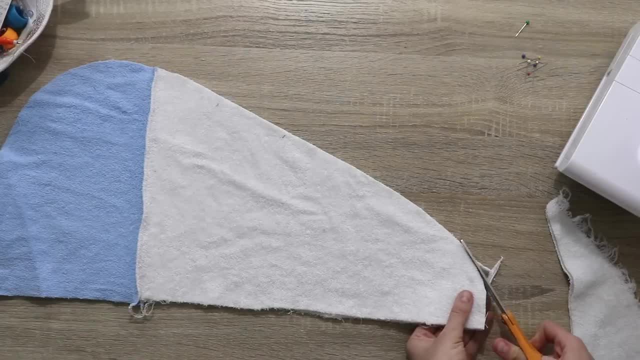 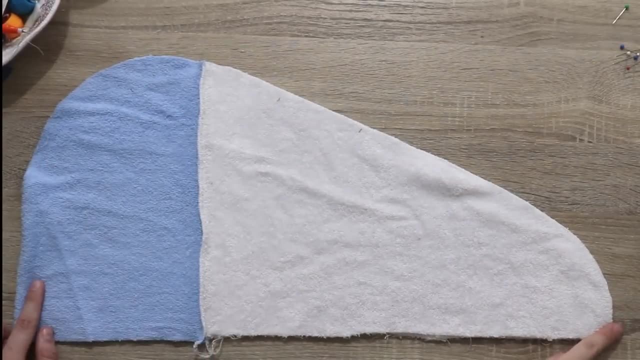 Now, even with doing my best, I was a little bit short on fabric, so I hope it still fits well. When sewing the top seam, I have to insert elastic on one side, and I didn't have small elastic, so big one it is. 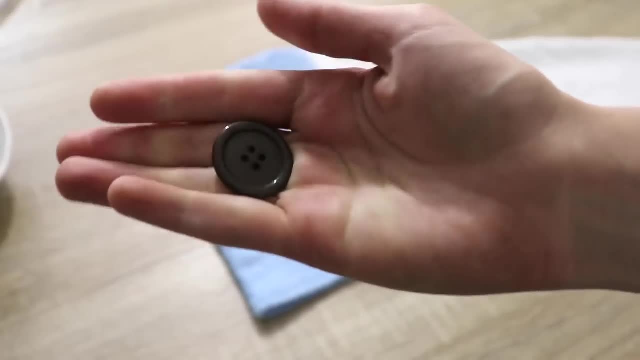 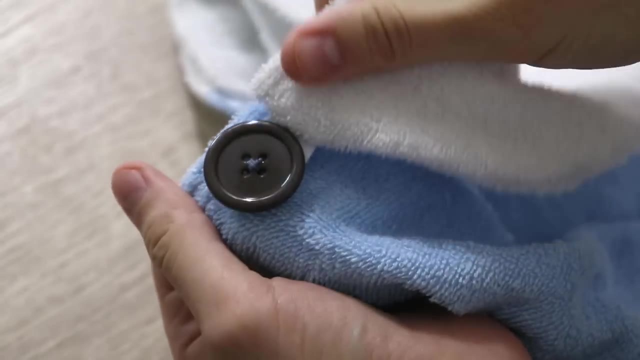 Then of course, you have to hem it and attach a button on the opposite side of the elastic, And again, I didn't have a matching button. so it is what it is. Overall, this project is really easy and again, I have a full tutorial on my channel. 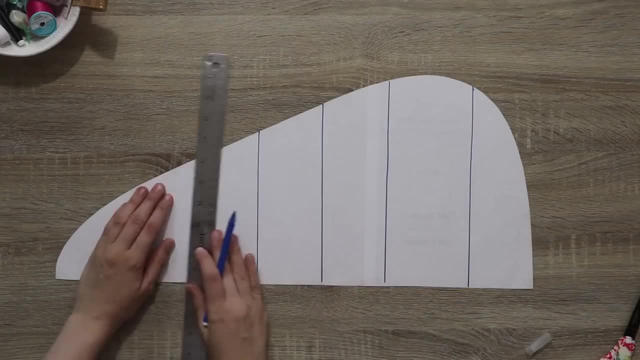 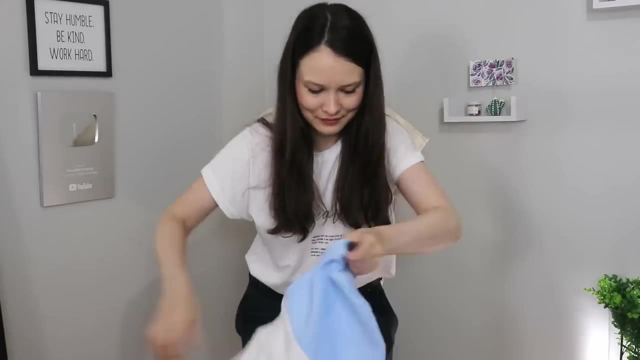 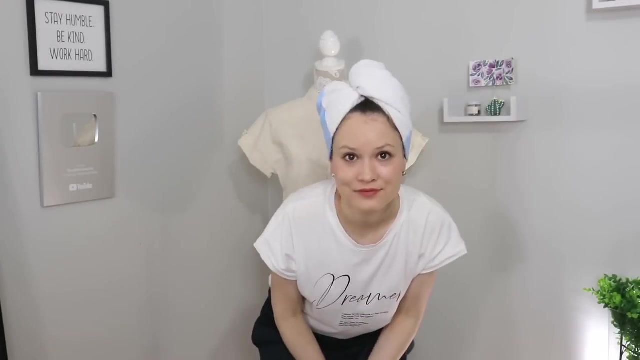 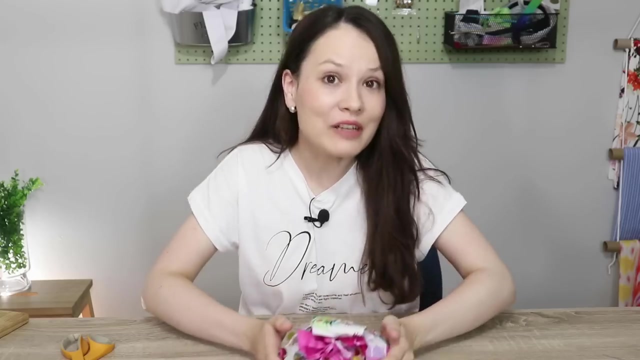 Now, if you have longer hair than I do, then you can use a simple slash and spread method and make the pattern longer for your needs. And now let's get started. Let's take a look at the final result. I really love this next idea as well, because not only it's great for little fabric scraps, but 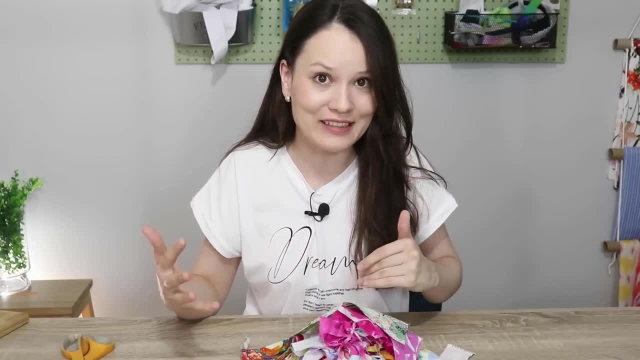 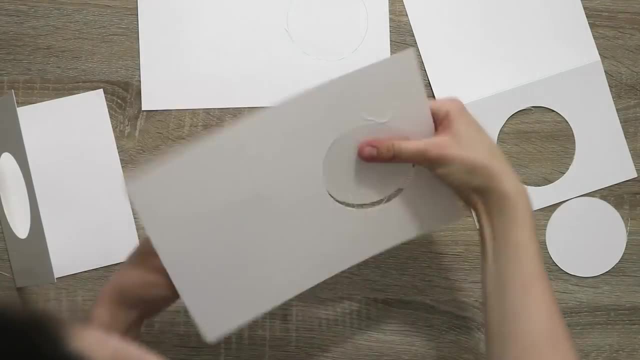 I personally also love to combine sewing and art. Here I'm starting with cardstock or watercolor paper that I folded in half to make it into a card and a circle cardstock. So I'm going to cut out a circle in the middle. 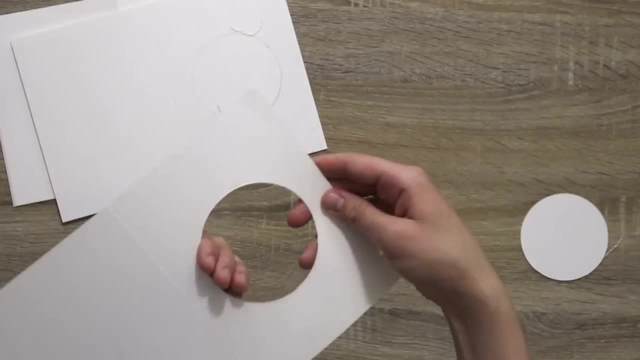 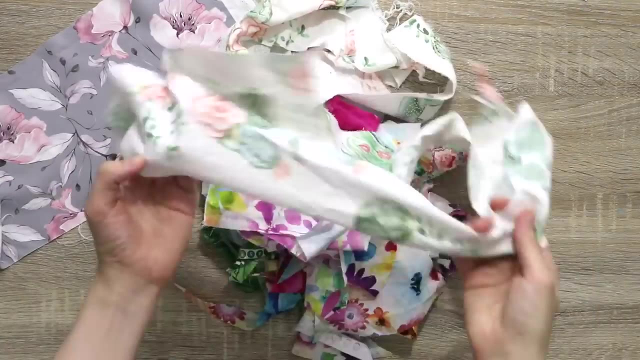 And of course, it doesn't have to be circle. You can go for square triangle or any other shape that you would like. Now grab your beautiful fabric scraps and have fun. What I do is I try to find beautiful little pieces of print that would fit really well. 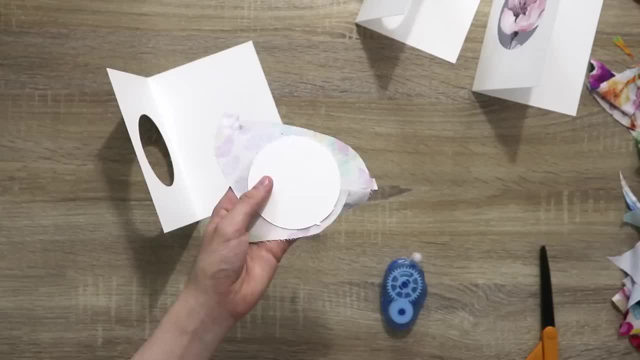 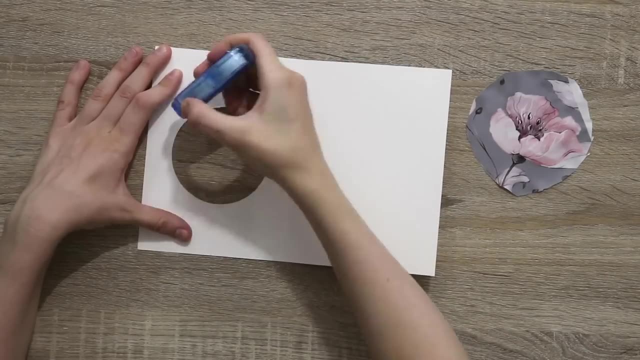 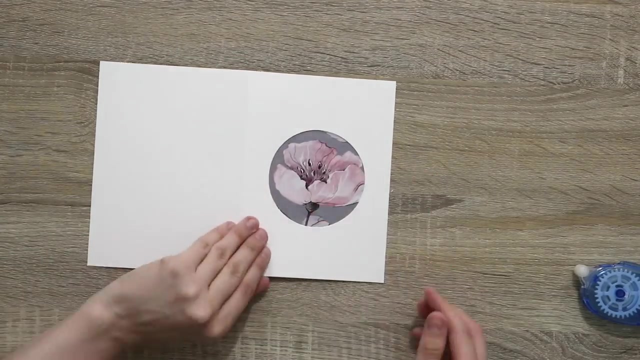 within that circle that I cut out in my cards Sometimes, when I have those gorgeous fabric scraps that I really don't see using in any other projects and they're just too tiny. I feel that this is a really good idea. I feel that this is a really great way how to have fun and also brighten somebody else's day as well. 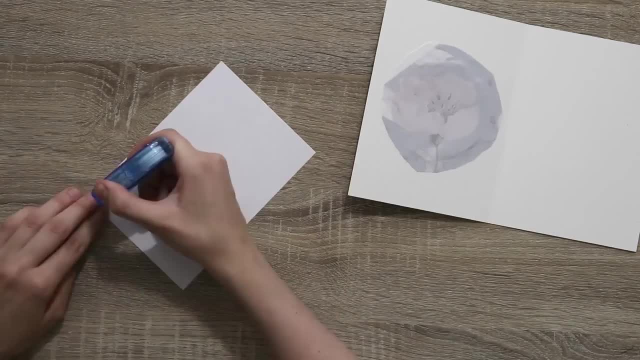 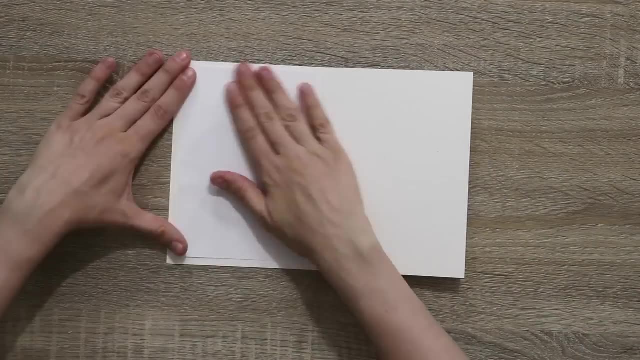 Once I have glued my circles down, I usually take another piece of paper, a lighter one, like a printer paper, and then I tighten up that back side, so that way it looks nice and neat. Now, of course, you can leave it as is, but in my case I like to take out my watercolors and 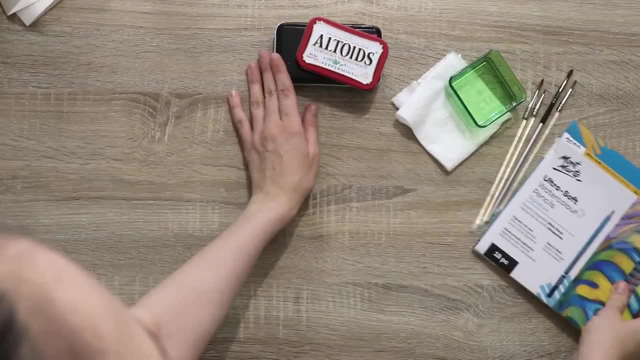 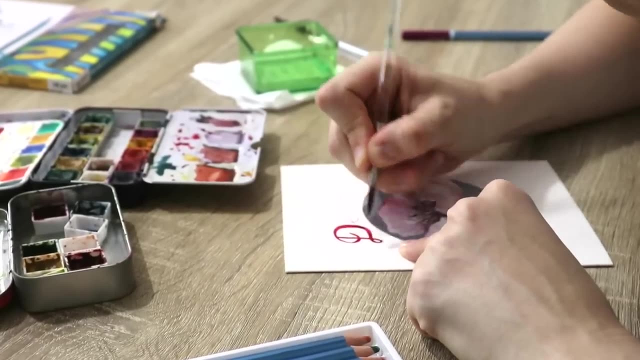 my watercolor pencils and add a little sentiment and, just, you know, a couple of splashes of color here and there, just to bring it all together. So I'm going to paint that back here. This is the end of the video. 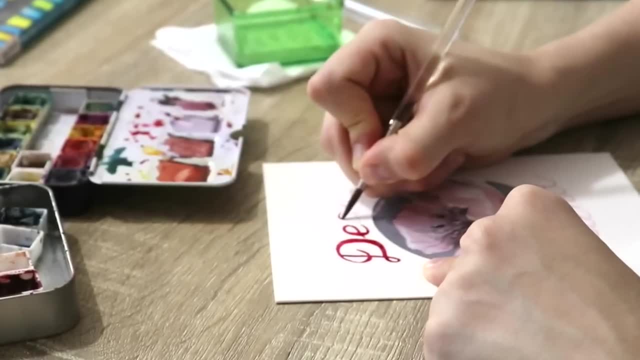 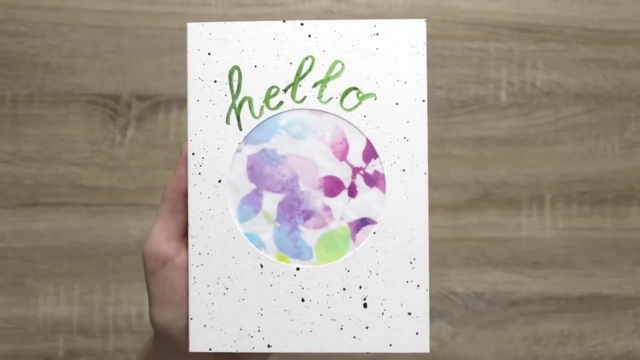 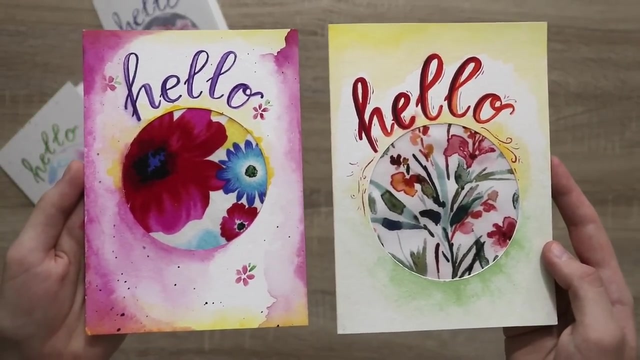 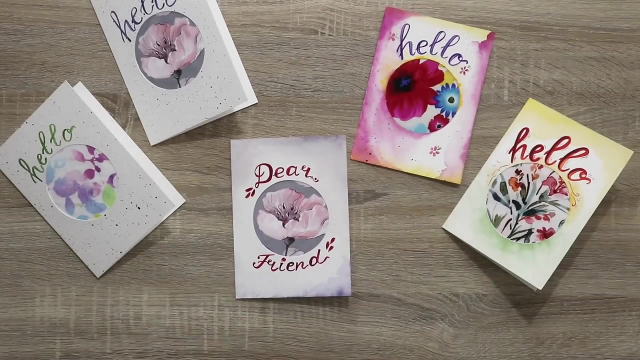 I hope you enjoy it. Like and share this video with your friends. You can find me in the description. I'll see you in the next video. Thanks for watching. I'll see you next time. Bye, For this next project. I will finally use up this blue linen scrap that I had no. 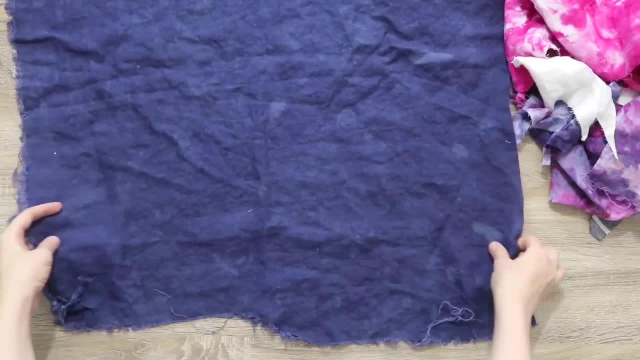 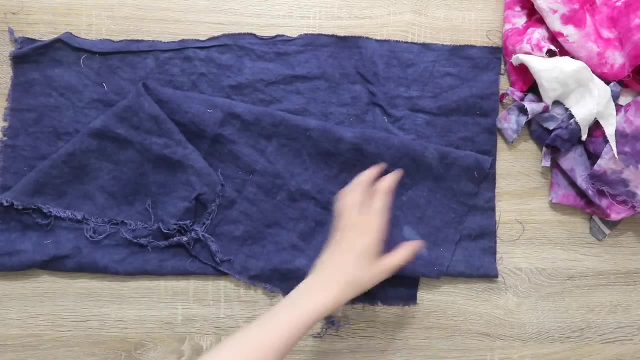 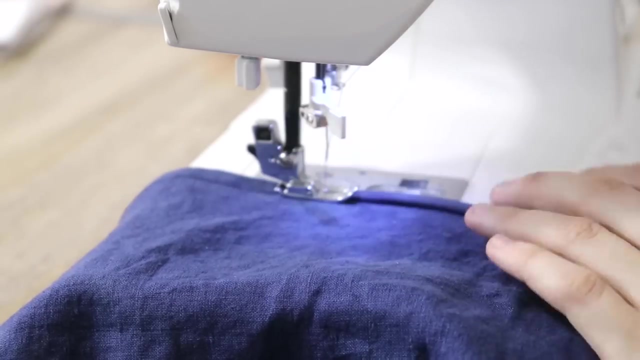 home for a really long time. So let's make kitchen its home. I'm going to cut it about 25 by 18 inches, and that's approximately the size that I cut all my linen towels From here. I just have to hem all four sides and that would be it. 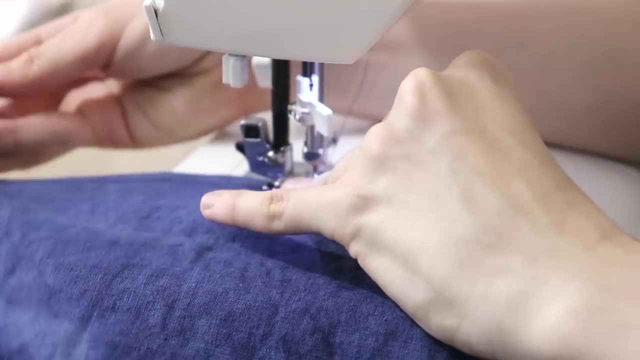 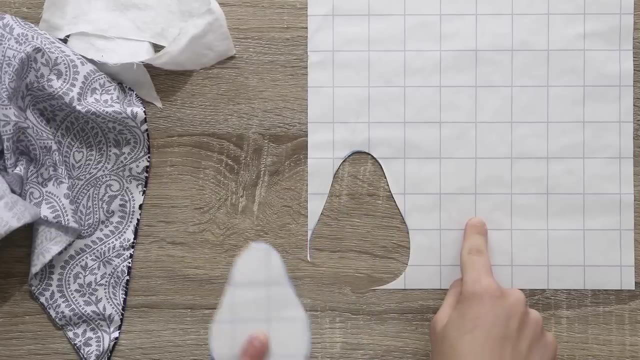 But I also want to try something new. So recently I picked up this double-sided interfacing for applique, So let's give this a go Now. fruits come to mind when I think of kitchen and tea towels, So I will start by cutting a silhouette of a. 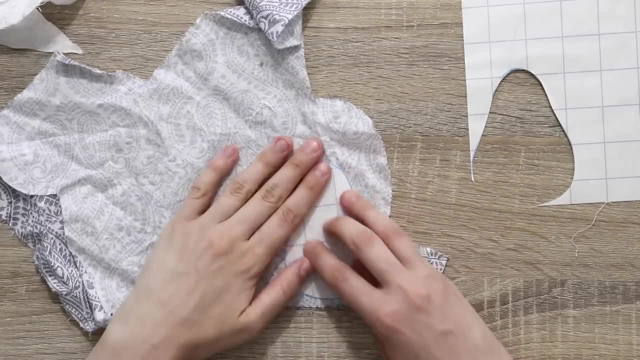 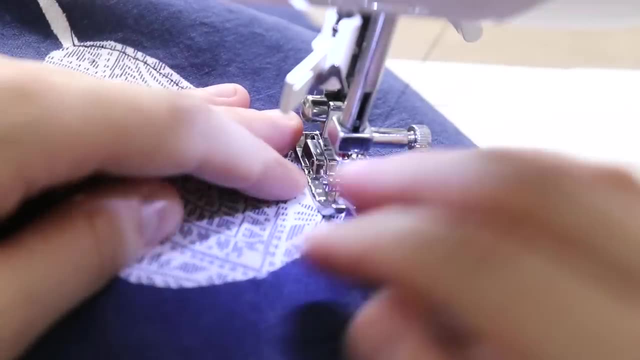 pear, and, following the directions on the package of this interfacing, I first fuse the shapes to the linen towel and then I topstitch them. However, I'm not a fan of doing raw edge applique and as this is a linen towel for kitchen, it's going to be. 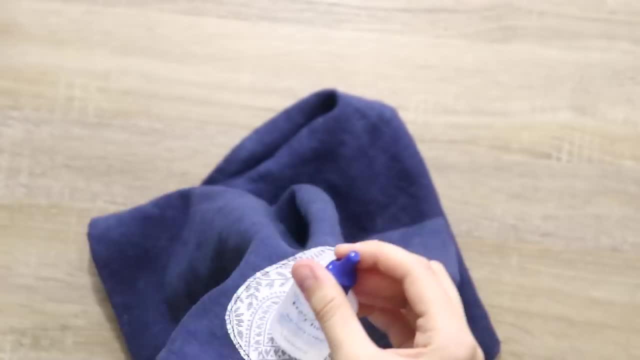 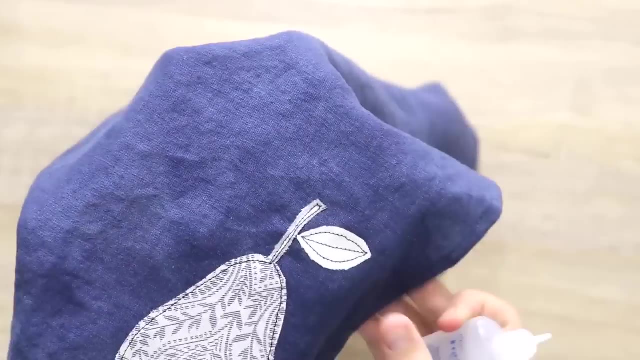 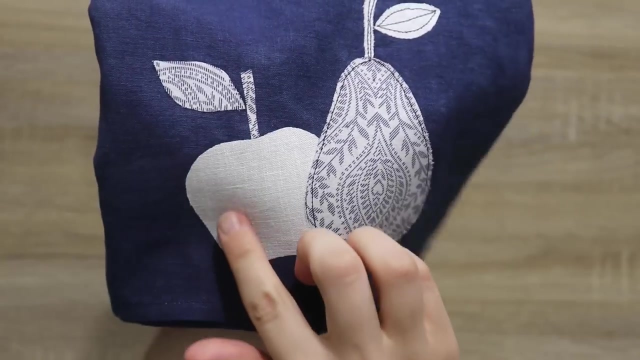 used quite a bit, So I wonder how it's going to turn out. So, in order to prevent really excessive fraying, I'm going to use fray check on the edges of the pear. After looking at it for a little while, I decided that that pear looks a little bit lonely, so I added an apple to keep. 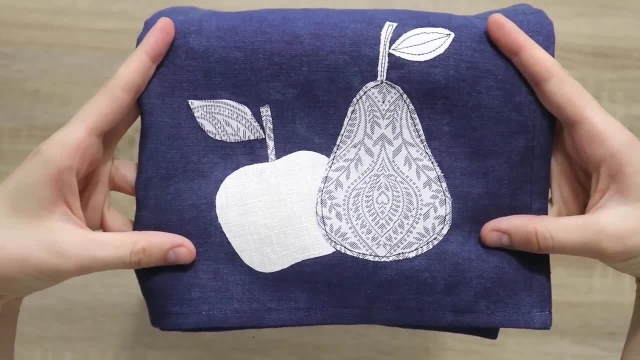 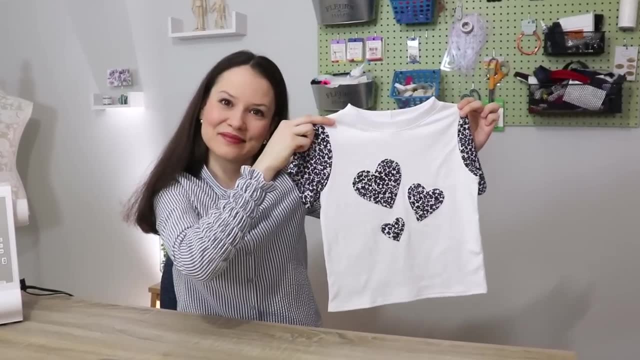 it company For the apple. I decided to not to topstitch that as a part of the experiment because I wanted to see how well this interfacing is going to hold up. Needless to say that you can use this technique not only on kitchen towels, but 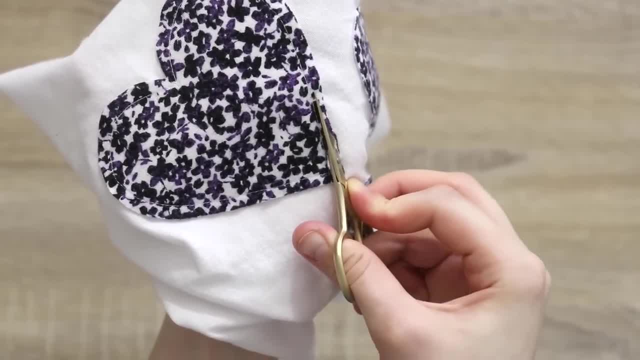 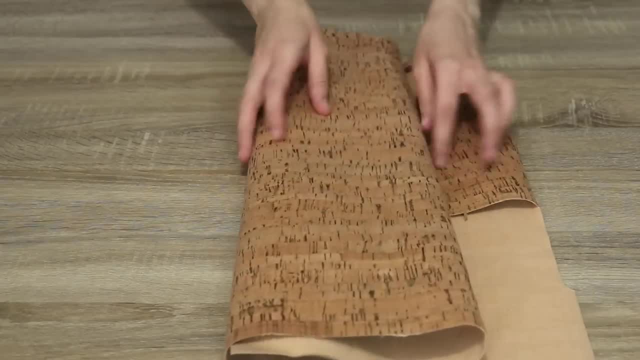 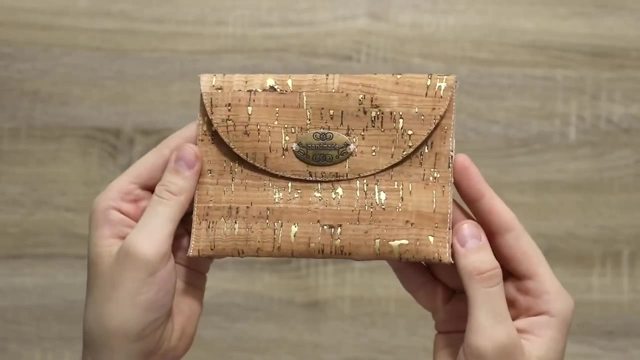 also on a variety of other really fun and exciting sewing projects. Next up is this piece of cork fabric that I had for quite some time, and originally I bought it to make these little mini wallets that I made as gifts, and they were a huge success, and I want to basically make a larger version of that in order. 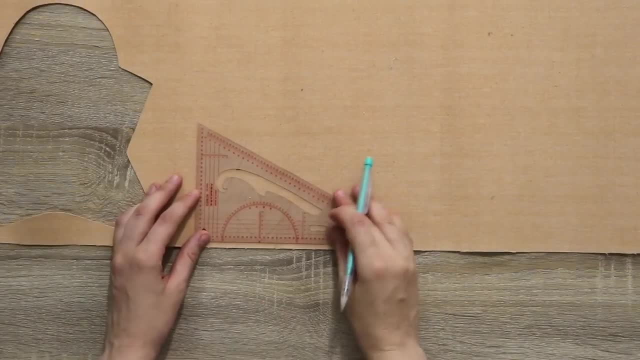 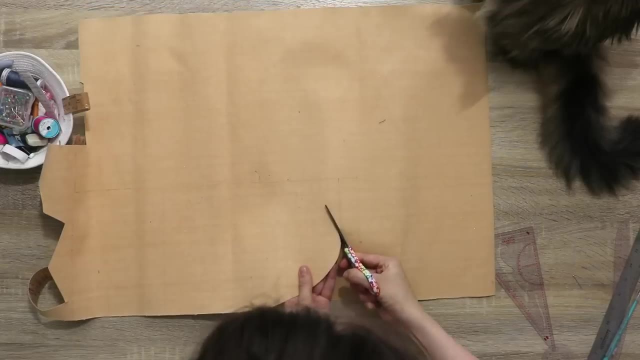 to be able to carry my travel documents all in one place. I'm going to draw and measure my template right on the cork fabric, because it's literally just a rectangle with slightly rounded edges, and that's about it. I do, however, want to add a pocket on. 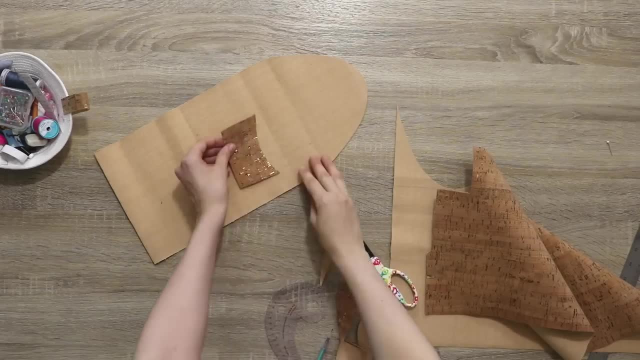 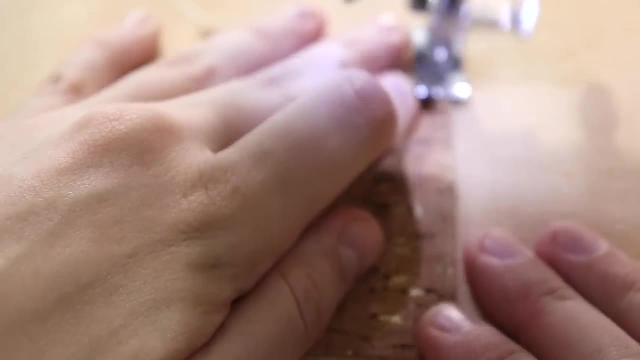 the inside as a card holder, and that is the first thing that's going to be attached. The beautiful thing about cork fabric that it doesn't fray, so this project really comes together super quick. After that, I just fold up the bottom onto the middle part and stitch it again. 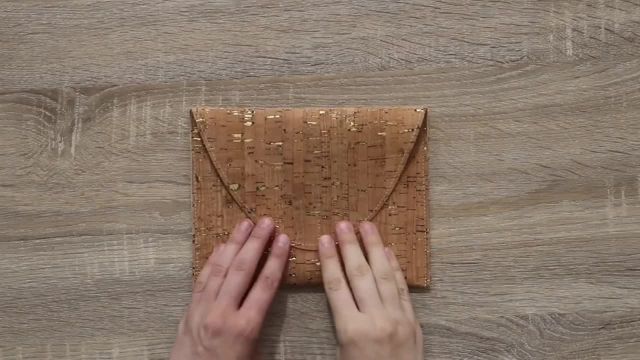 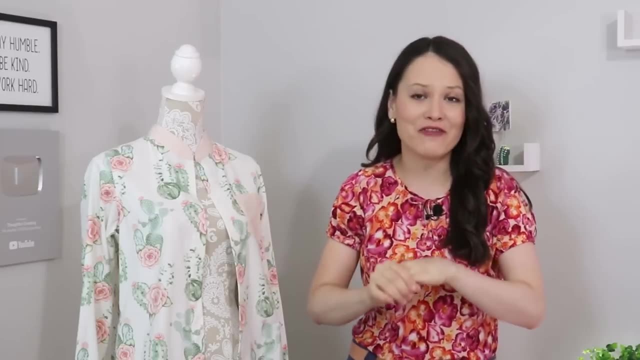 The last step is to add a little closure, and that's it. your document organizer is done. Now here are 10 of my best tips on how to work with fabric scraps, how to combine fabrics, how to find grain line and all of the